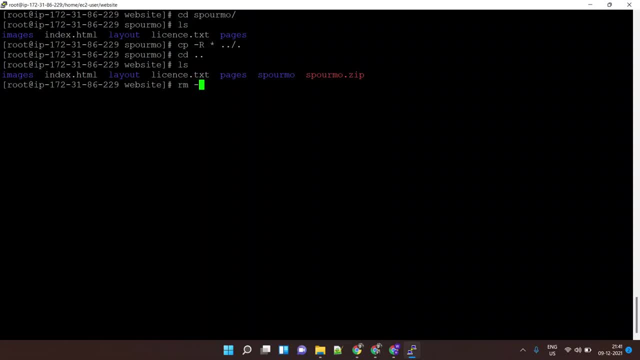 the necessary files. let me remove the redundant zip file and the folder which got extracted from the zip file. that is gone now, so we have the necessary pages or necessary html site. now i want to run this html website, okay, inside a container, not directly, by installing an. 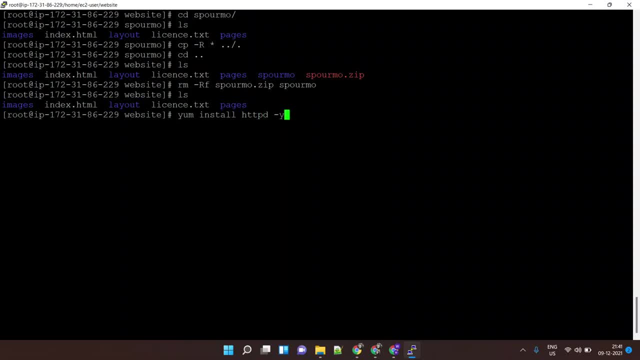 apache web server. so i can simply do an http install. uh sorry, m install httpd, hyphen y, and this will install apache web server on the ec2 instance itself. so i don't want to do that. i don't want to install any web server on this ec2 instance. what i want is i should have a. 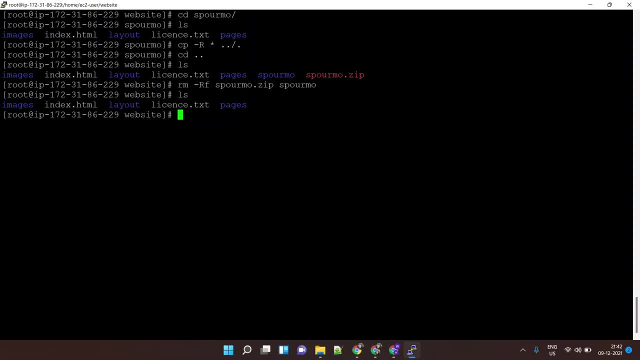 container and inside that container there should be an? uh, there should be httpd installed and on top of this can, on top of that container, i want to run this website. now, uh, what you can do is you can uh create a docker file for this and inside your docker file, you can start from any base. 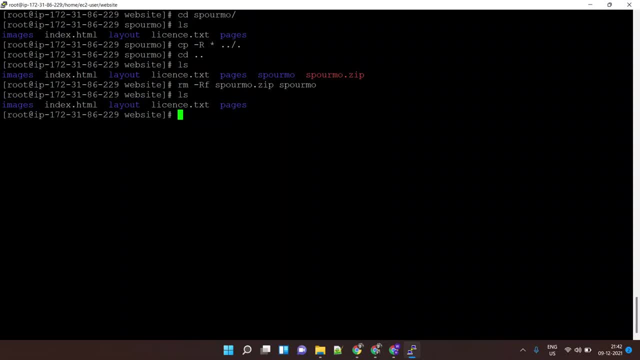 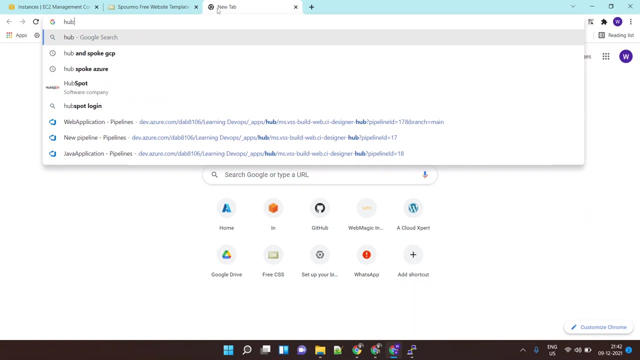 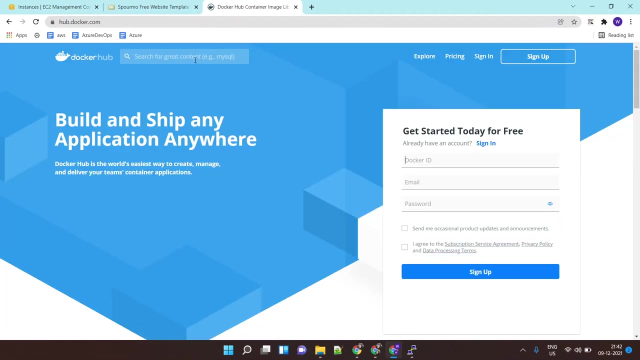 operating system and on top of that base operating system you can install apache and then copy all these files inside that, uh, inside that docker image. that's one approach. or else you can simply go to docker hub by going to hubdockercom, and over here you can search for httpd and over here you will find an readymed image for. 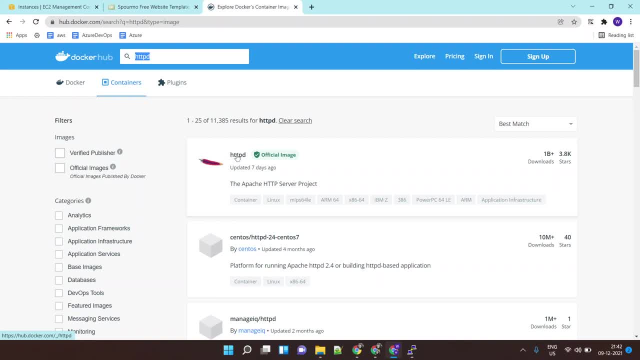 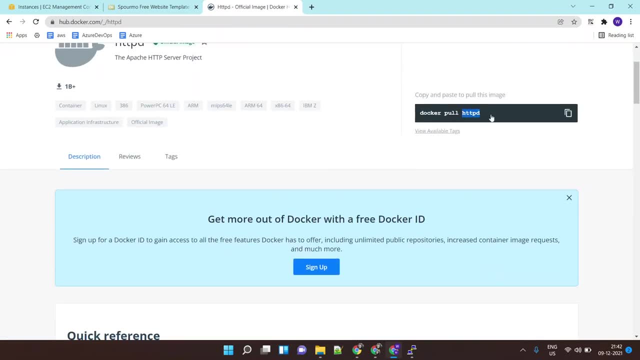 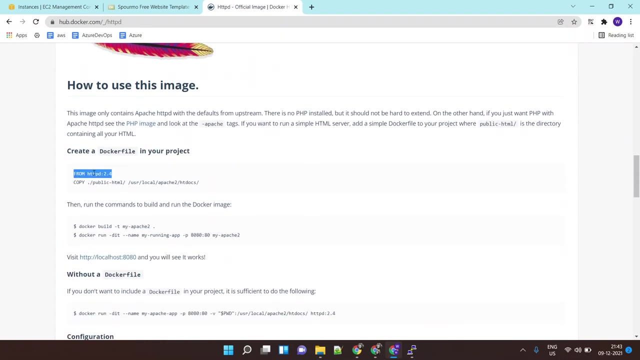 an httpd, so this means you don't need to install httpd. this image comes pre-installed with httpd, so i'll get the name of this image. so the name of this image is httpd itself, and what i would need to do is i would just then simply need to create a docker file which will 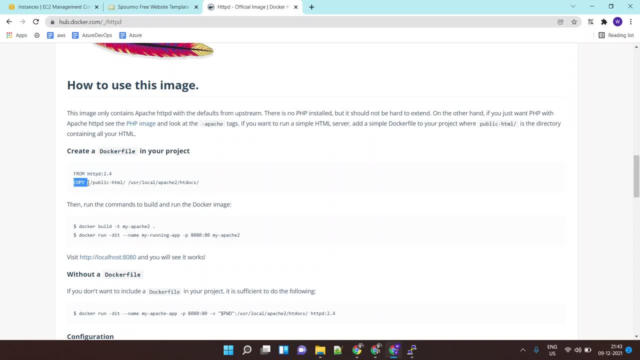 have the images of theuftdocker rather than the Schüler file, which will have the image on the bikini image also, and also the docker file is an image, when i just I just simply need to create a docker file reference httpd and i will need to copy all my files. which files these files right from my base. 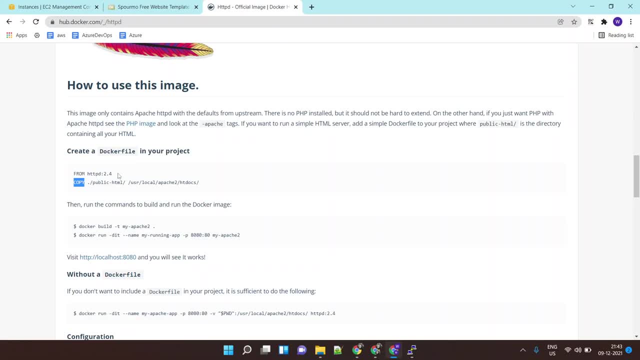 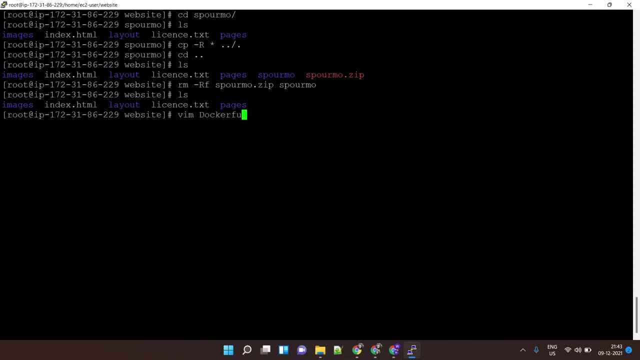 operating system inside the image itself. as an additional layer, let's try to do this inside docker file. so i'll say vim, docker file and over here first i'll say from httpd. this means it will download an httpd base image and on top of this base image what i want to do is i want to copy. 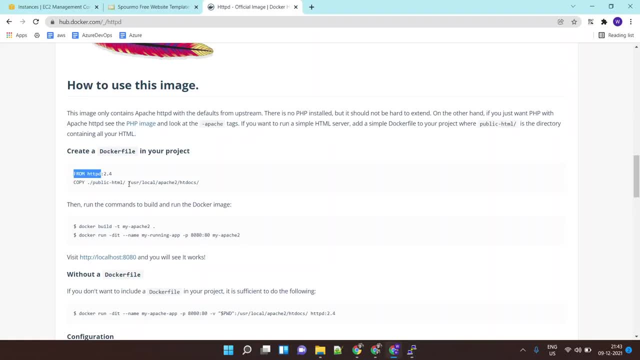 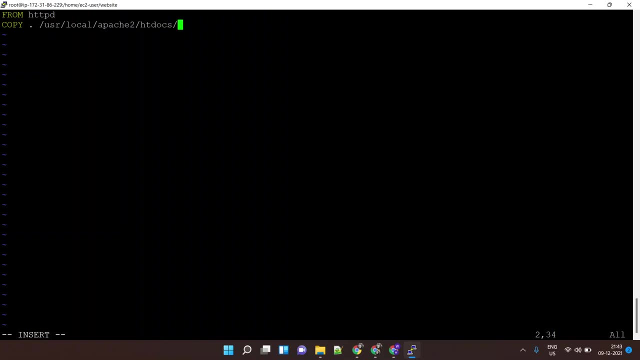 all the files from the current directory to a working directory of my httpd server, which is user local apache to htdocs. so all the web files should go inside this folder. that's all i need to do, and this will create an image for me which will have httpd with all the necessary applications. 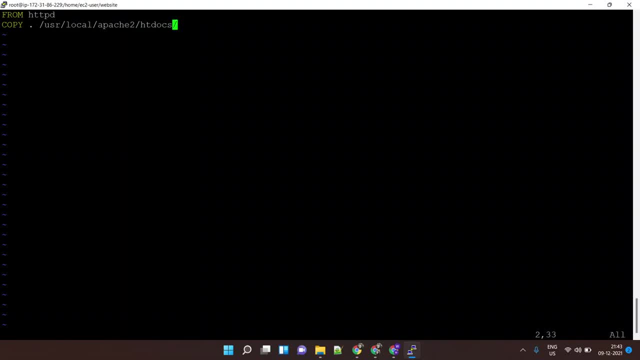 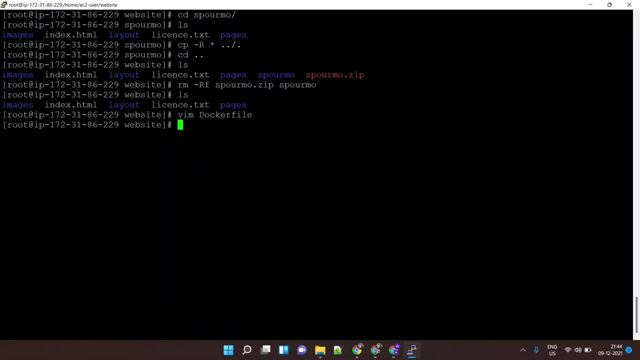 so let's see how it looks like. let me save this image. so we'll save this file, and now i'll say: docker build. let's tag this image as website by hyphen t. so let's do a dot. dot means current directory. there is a docker file using a docker. 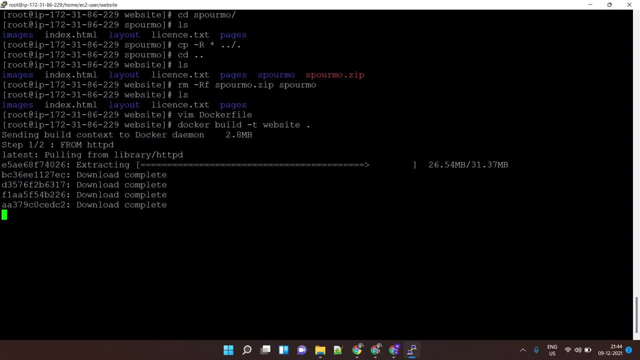 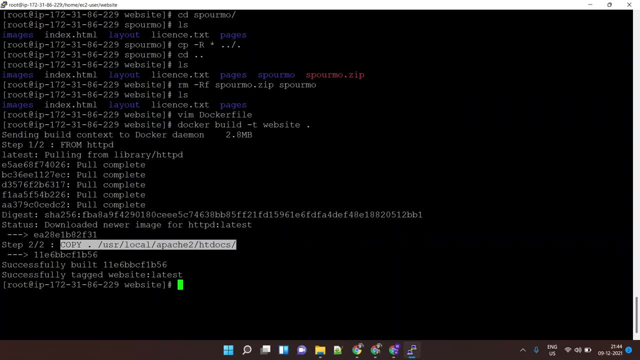 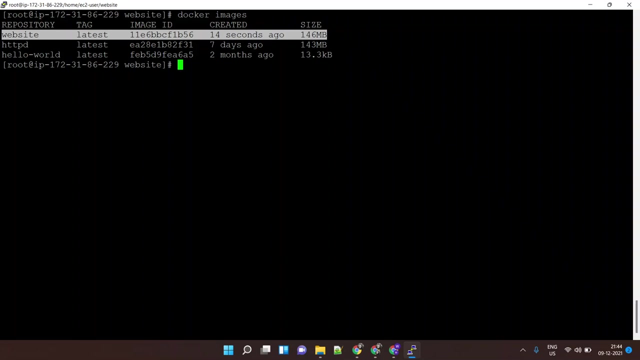 file build an image. here we go. it is downloading a download, downloading httpd image and then it is copying all the files from current directory inside the http side of folder, which is user local apache to htdoc. this means that the image is ready. so i do docker images. now i'll have image ready over here. now i can run and i can create a container. 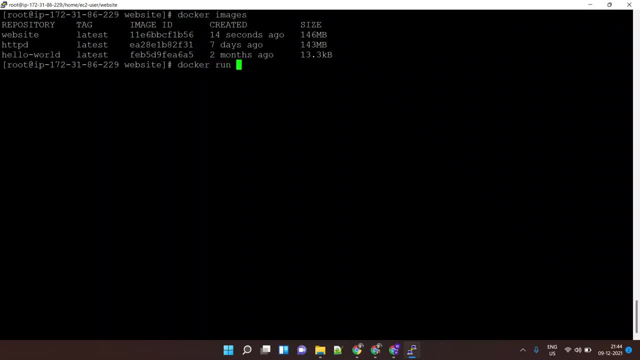 running container from this image. so for doing that, i'll say docker run. i want to run this container in, uh, let's say background. okay, i want to run this container on port number 80. i'll say 80, 80. so the container port and the host port. 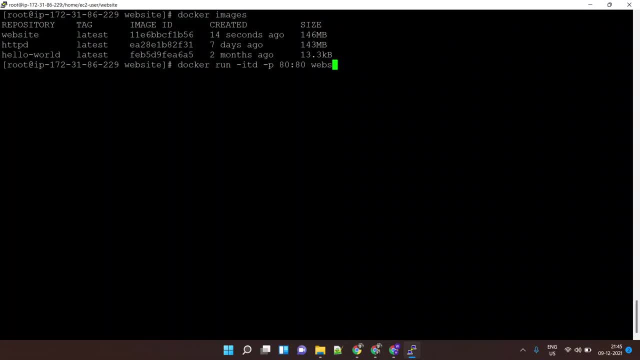 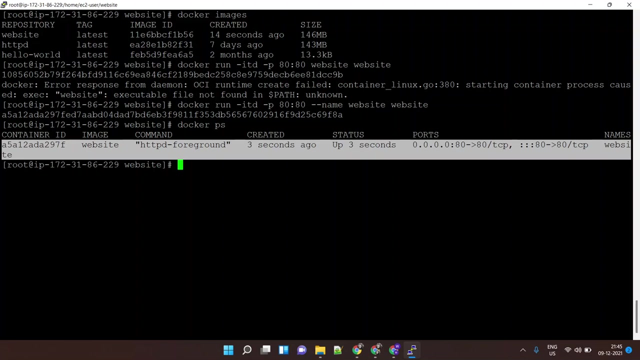 and i'll say the container name as website, and it has to be created from an image known as website. okay, that will do the work and if i do docker ps, let's see a running container over and i can also access this container or the website running inside this container. 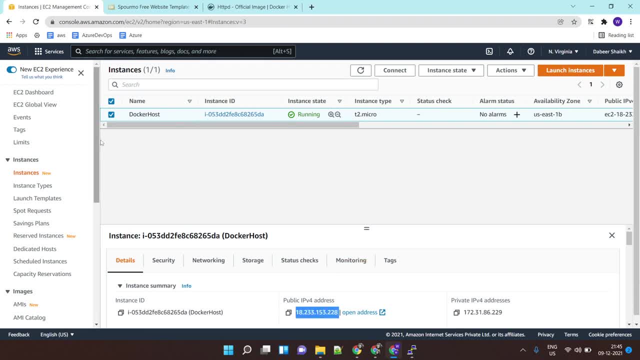 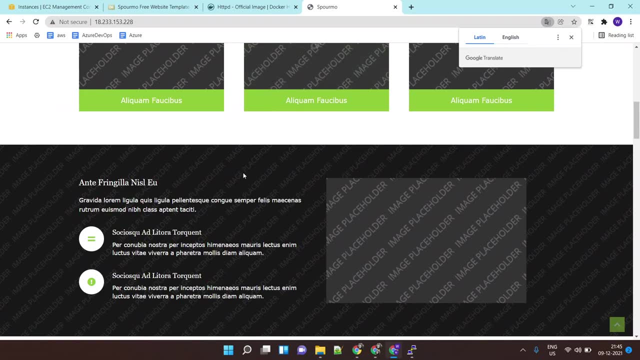 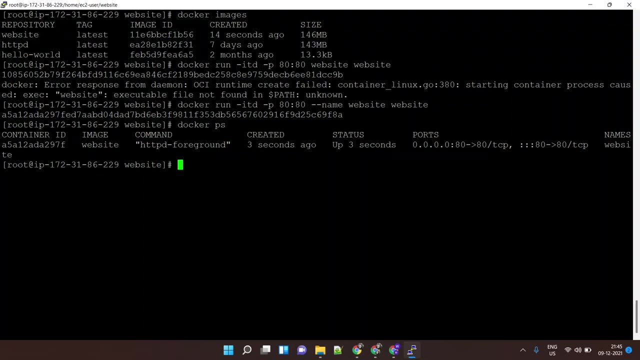 over a web interface. so if i copy the public ip of my docker host and i would be seeing a website, html website running inside a container on the ec2 instance. so this is how you can create a very simple docker image, very simple docker file. this is it for this. lab guys. thank you for watching.